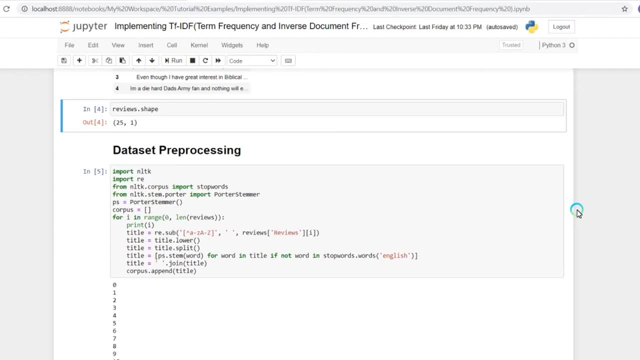 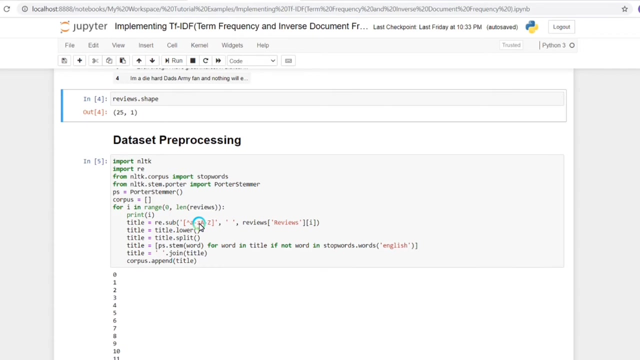 Text that is present, our dataset, into some proper format, That which can be applicable for vectorization. So for that, what I did is I have executed a for loop for the, For the complete dataset, from 0 to the total length of the review. So here I am removing the special numbers characters present in my text or the reviews. 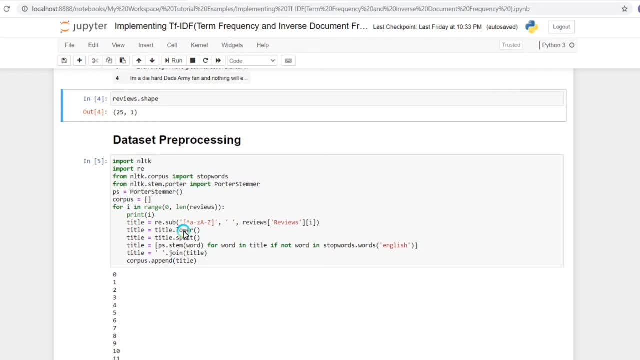 so after removing, I am converted into Converting it to lowercase and after that I have splitted all the words and checking whether the words are stop words or not. If it is stop words, I'm removing that word and other is I am keeping the that particular word. 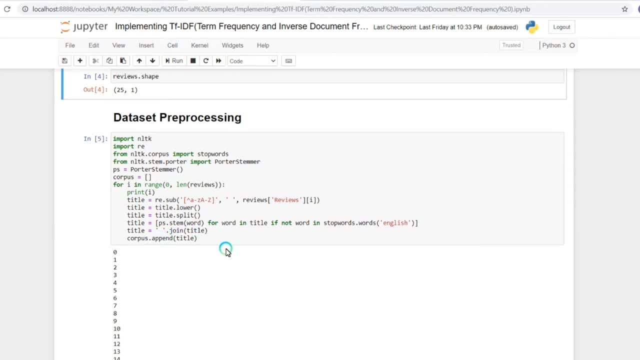 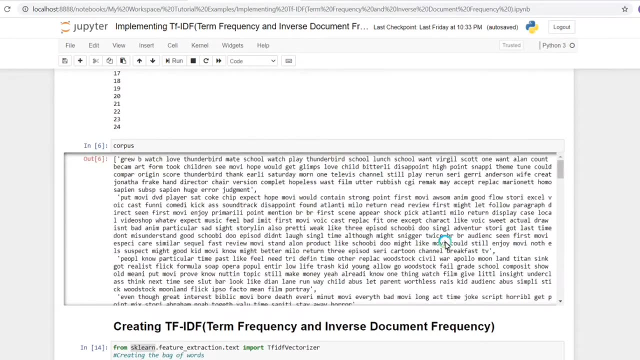 so, finally, I have added all the reviews into my corpus, like after pre-processing. so here we can see the corpus which contains all the words into some proper format, like we said, which can be applied to or which can be used to directly, directly to The TFIDF vectorizer to convert it into some satisfies form. 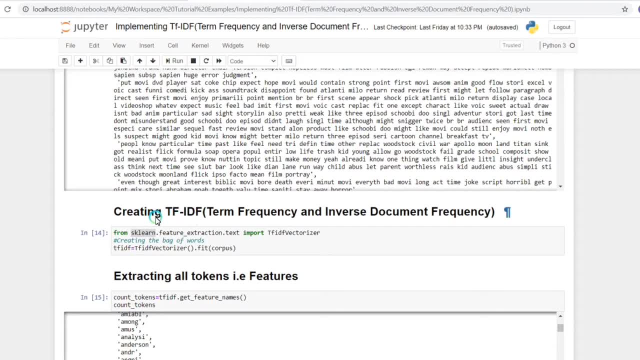 so here I am declaring the TFIDF vectorizer, vectorizer which I import from the SQL and library. so here I'm importing the tf-idf vectorizer from SQL and library and after that I am creating a tf-idf vectorizer. so here you can see. so after that I have created the tf-idf vectorizer. 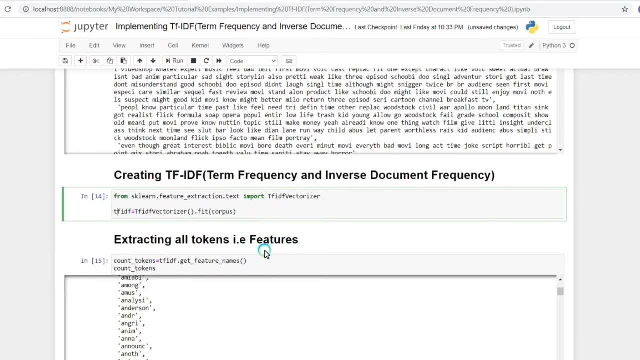 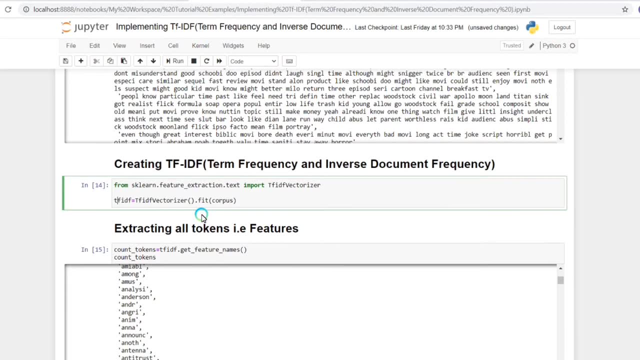 here. this is the model. so here I am fitting my tf-idf with the corpus. that is, that is it. so I have given the corpus to the tf-idf vectorizer, so after giving it, converts. it makes the model based on the corpus. so here I'm. 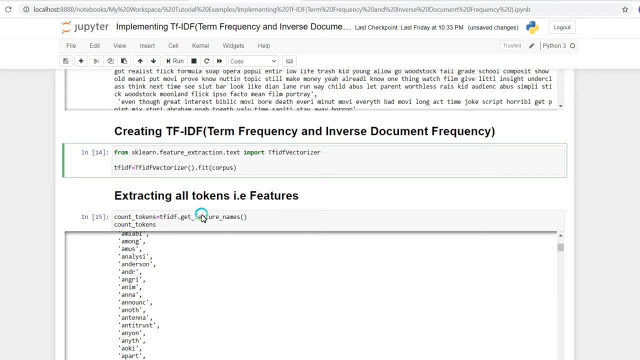 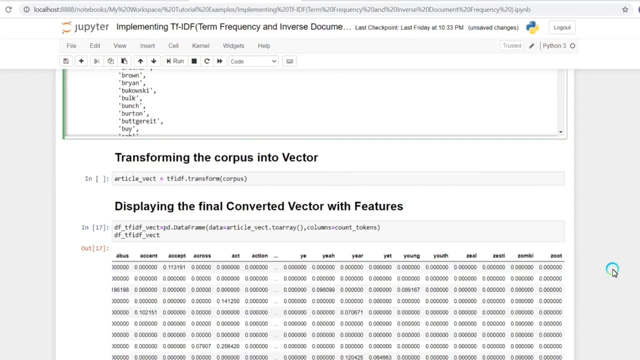 extracting different features or the different words that are present in my data set. so here I'm extracting the words using git feature names. that is is an inbuilt function of tf-idf. so here you can see all the words present in my data set. so after that I am. 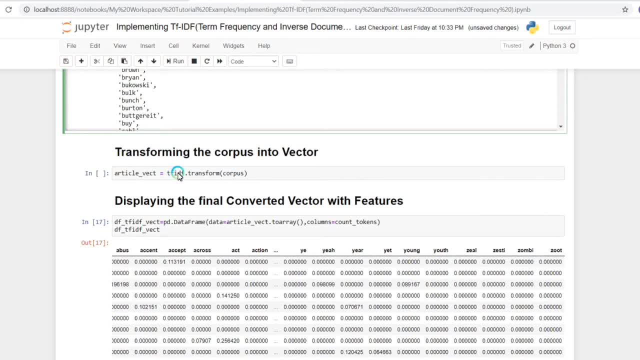 converting my corpus into that vectorized from. so here i can use the tf idf to transform, passing the corpus as an argument. you can see, i can convert the text into the vectorized from. so i have converted all the text into vectorized from and named this as.